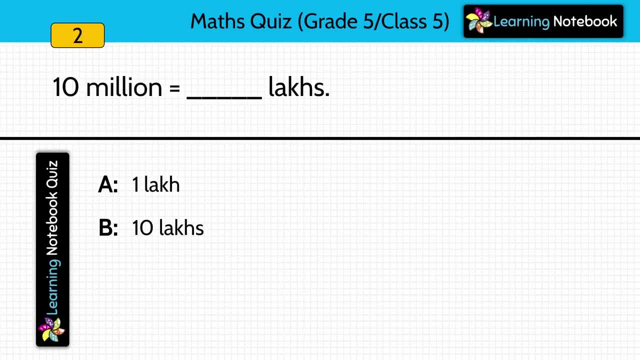 Next: 10 million equals to how many lakhs? Is it 1 lakh, 10 lakh, 100 lakhs or 1000 lakhs? Answer is option C: 100 lakhs. 10 million equals to 100 lakhs. 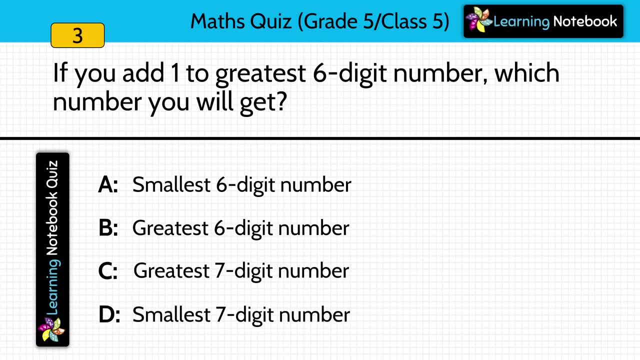 Next, if you add 1 to the greatest 6-digit number, which number you will get? So here, first you need to know which is the greatest 6-digit number and then you add 1 to it. Answer is option D: smallest 7-digit number. 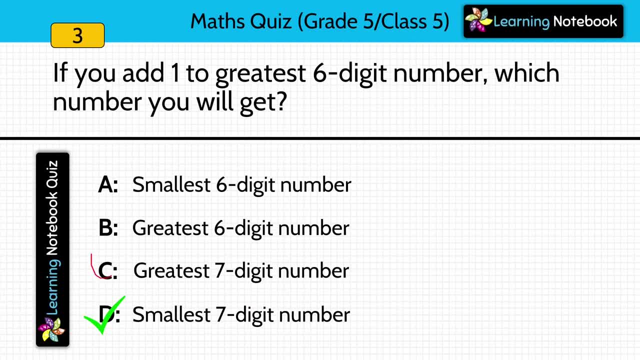 So how did we get this answer? Basically, first, we wrote the greatest 6-digit number, which is: this is 6 times 9.. This is the greatest 6-digit number Right Now. you will add 1 to it. 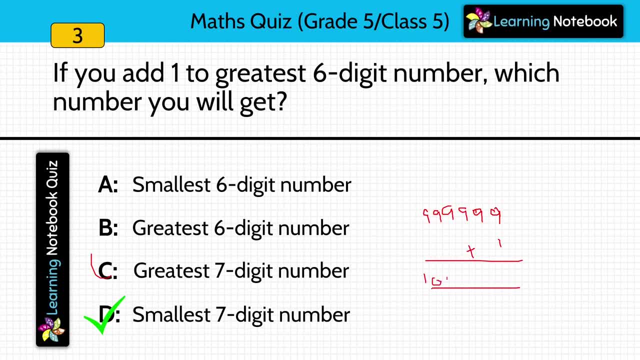 So what did you get? You got 1,, 2,, 3,, 4, 6.. You got this Smallest 7-digit number 1, followed by 6 zeros. So this is how you will solve this question. 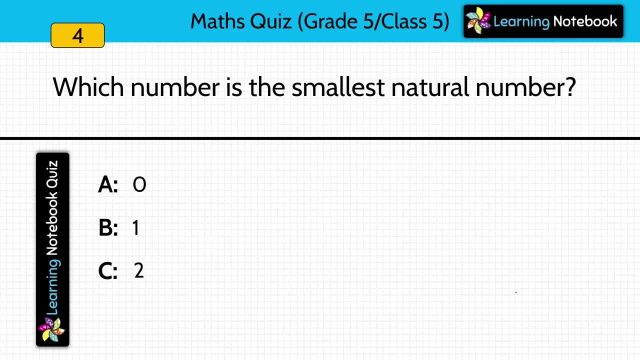 Next, which number is the smallest natural number Natural number? Smallest natural number Natural number? Answer is option B, 1.. Because? Because we know natural numbers are counting numbers and we always start our counting from 1.. Whole numbers start from 0.. 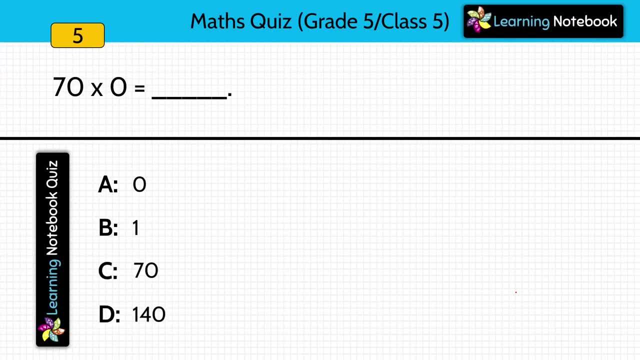 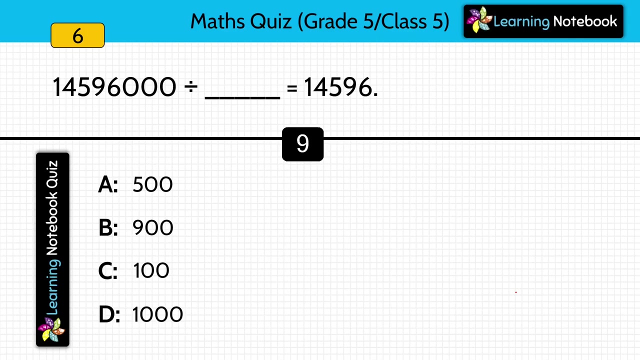 Next, 70 into 0 equals to dash. Answer is option A: 0.. Any number multiplied by 0, gives the answer as 0. only 14596000 divided by dash equals to 14596.. Answer is option D: 1000. 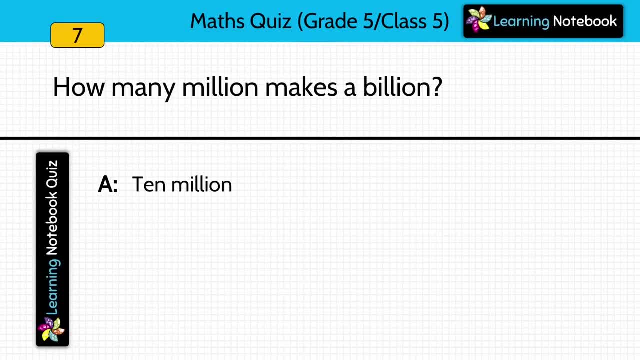 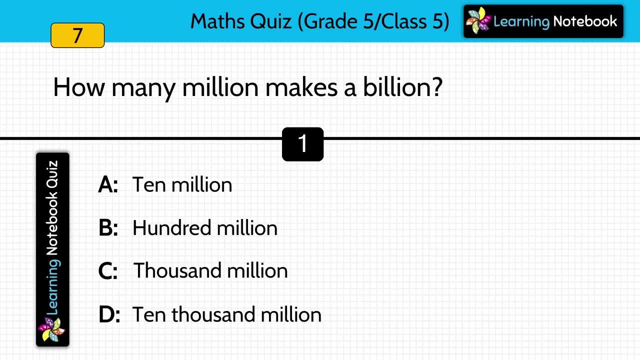 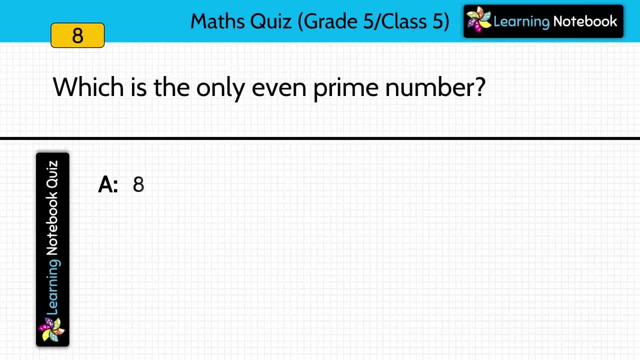 Which is the only even prime number. Look at the options. The answer is option B, 2.. 2 is the only even prime number. So what are prime numbers? Numbers that are divisible by 1 and itself only. That means they have only 2 factors. 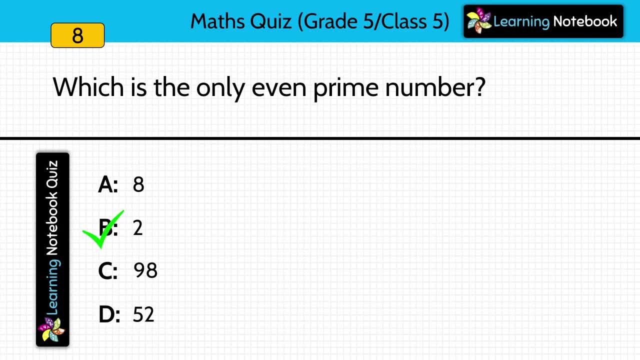 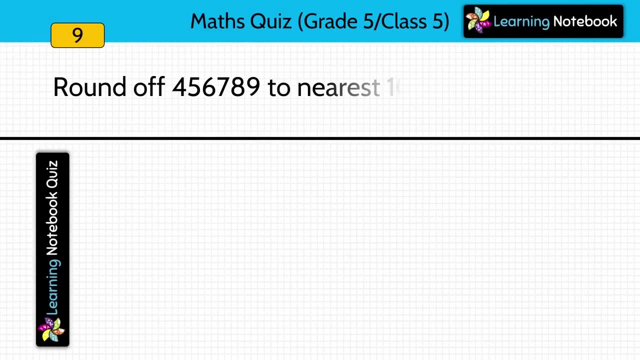 1 and itself. So 2 is the only even prime number. Other prime numbers are 3,, 5, 7 and many more. Out of them, only 2 is the even prime number. Round off this given number to nearest 100.. 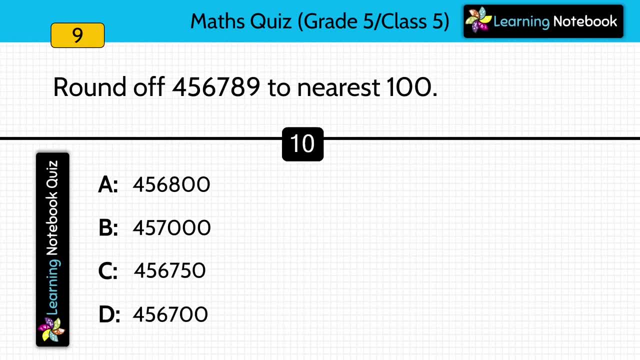 Look at the options You have to round off this number to nearest 100.. What will be the answer? Yes, answer is option A, 4,, 5,, 6, 8, double 0.. This is the answer. 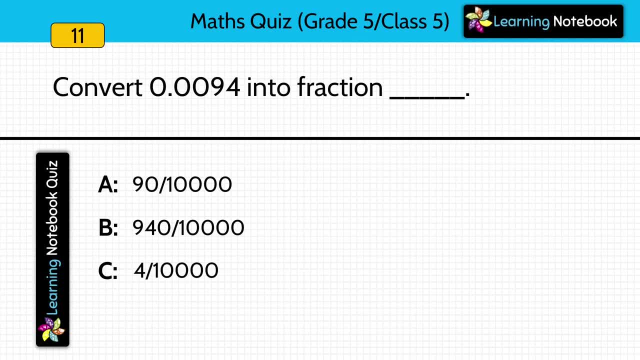 Next question: Convert 0.0094 into a fraction? This is a question regarding converting decimals into fractions. Answer is option D: 94 by 10,000.. Students, if you want to learn how to convert a decimal into fraction, you can refer to my separate video. 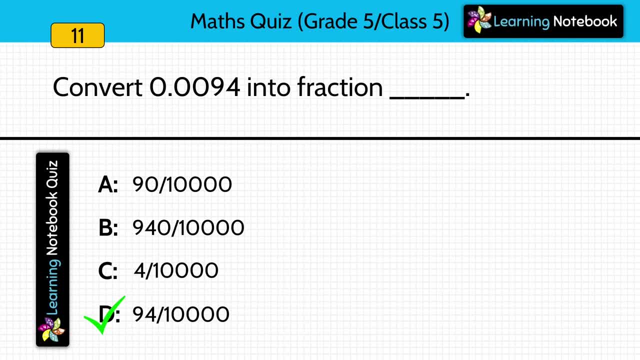 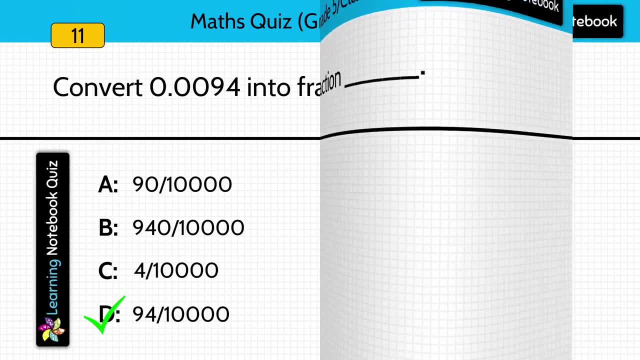 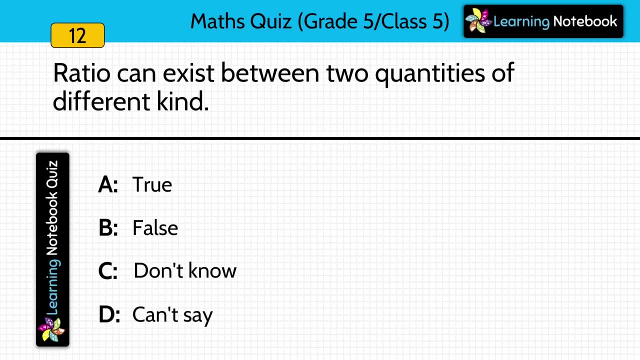 I would like to tell you that I have made videos on each and every chapter of Class 5 Mathematics, So do check out my channel Learning Notebook. Next, ratio can exist between two quantities of different kind. Is this statement true, false? don't know or can't say. 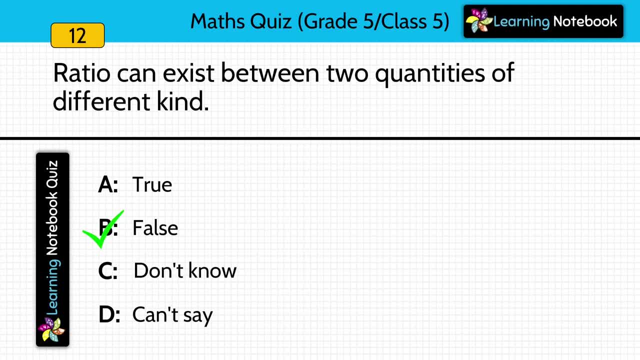 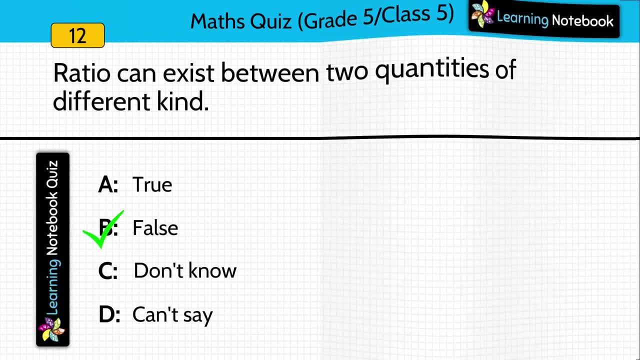 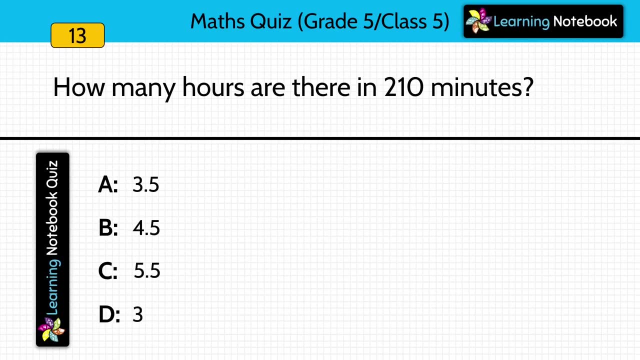 Answer is false. This statement is false. Ratio can exist between two quantities of same kind. How many hours are there in 210 minutes? How to convert minutes into hours? Answer is option A: 3.5 hours. We know that 60 minutes equals to 1 hour. 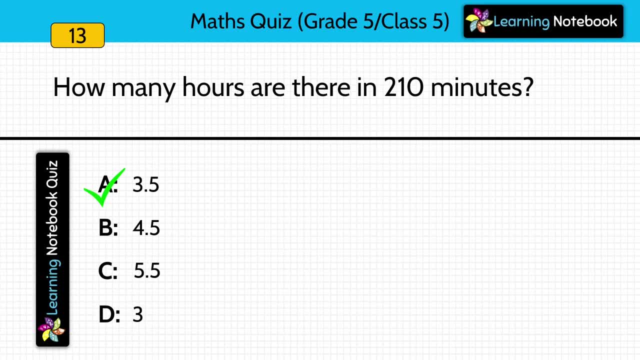 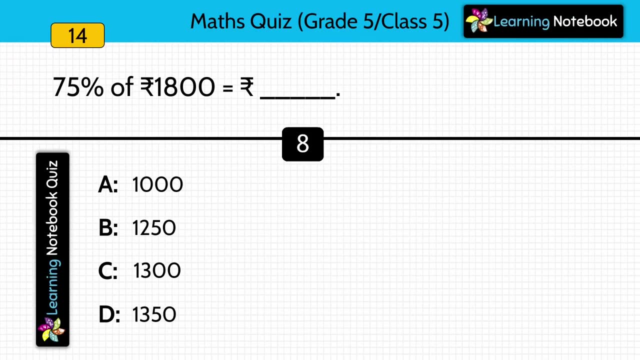 So 210 minutes equals to 3.5 hours. 75% of Rs.1800 equals to Rs dash. How to find a given percentage of a number? Yes, answer is Rs.1350.. How will we solve this? 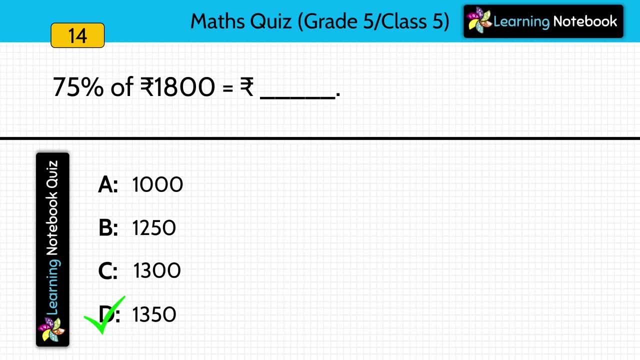 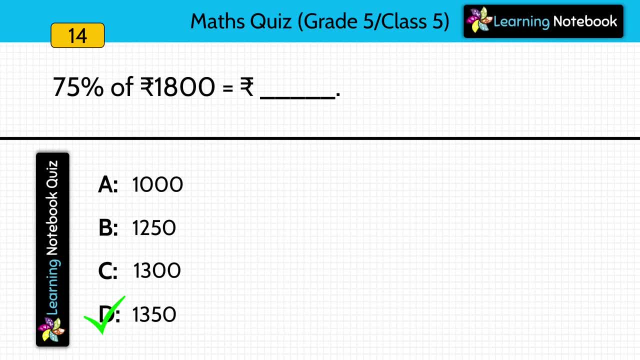 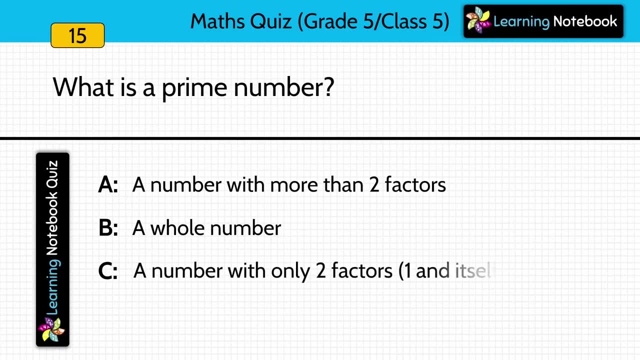 75.. 75.. 75.. When we solve this, we will get this answer as 1350.. What is a prime number Options? a number with more than two factors. a whole number? a number with only two factors. 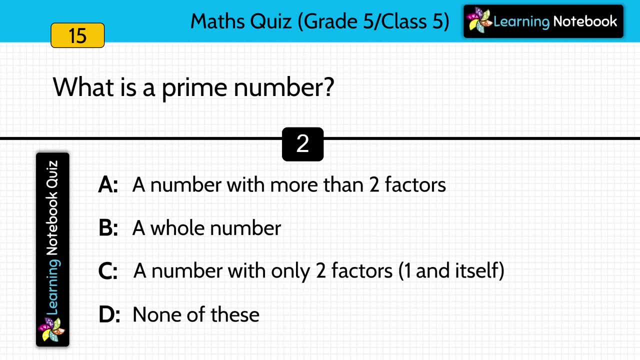 that is, one and itself or none of these. Answer is option C. A prime number is a number which has only 2 factors 1 and the number itself, For example, number 2,, 3,, 5,, 7, these. 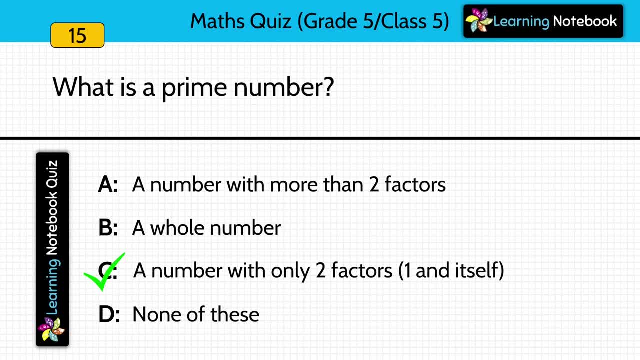 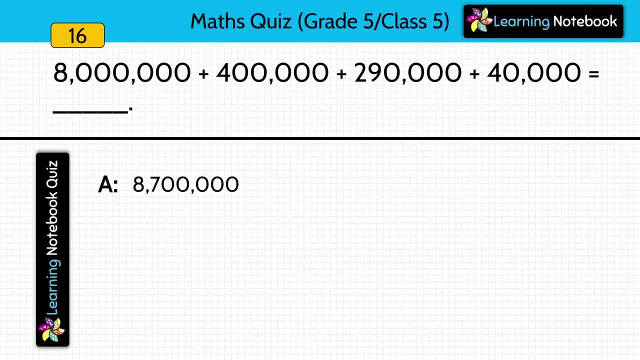 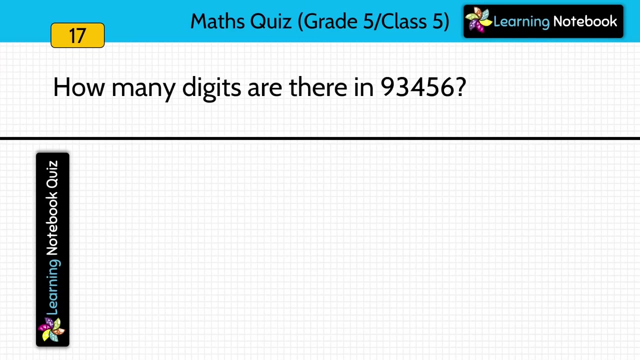 are prime numbers because they have only 2 factors: 1 and the number itself. We have to add these given numbers: 80 lakh, 4 lakh 2 lakh, 90 thousand and 40 thousand. Come on, add them fast. Answer is: 87 lakh 30 thousand. How many digits are there in? 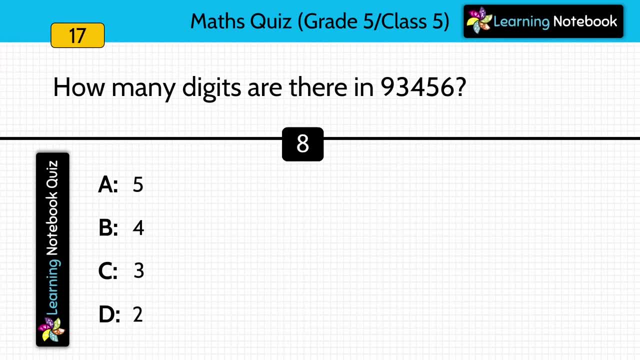 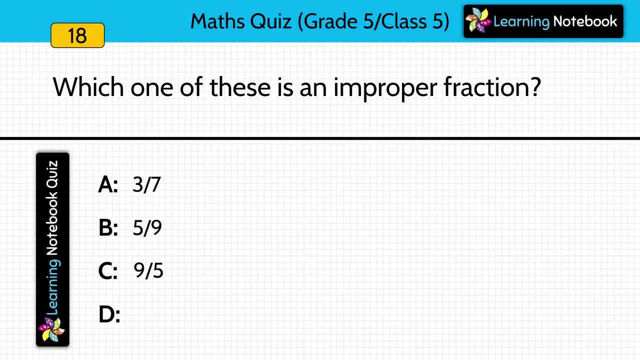 the total Number 9,, 3,, 4,, 5, 6.. Answer is: 5 digits are there? This was a pretty simple question. Which one of these is an improper fraction? Options 3 by 7, 5 by 9,, 9 by 5 or 4 by 11.. 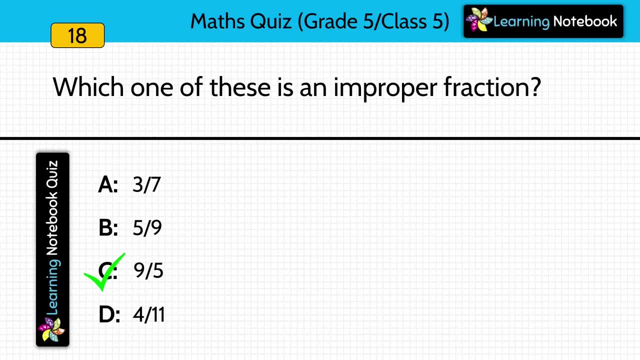 Answer is option C, 9 by 5.. So what are improper fractions Where numerator is greater than denominator? So if you look at the options here, you will see that, except C, all the other fractions, All the other fractions are proper fractions. 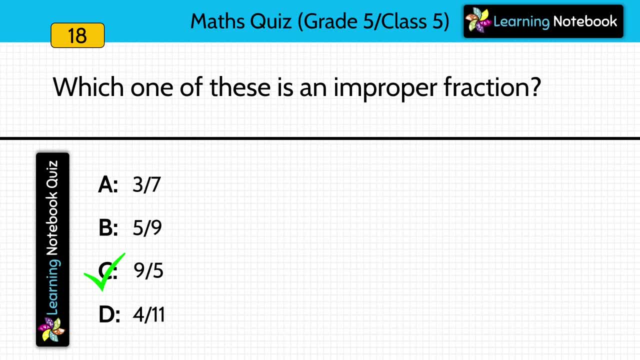 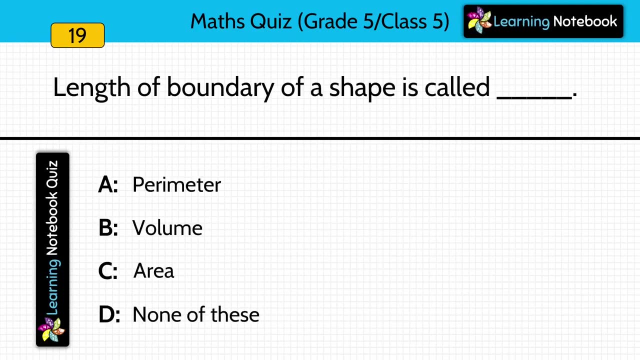 They have numerator less than the denominator, But 9 by 5 is an improper fraction because its numerator is greater than denominator. Length of boundary of a shape is called dash. Is it called perimeter, volume area or none of these? Answer is option A, perimeter. 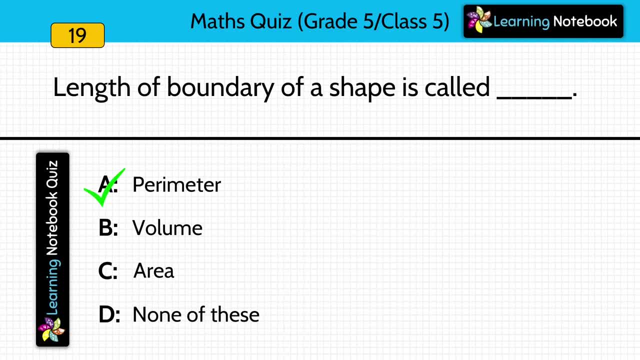 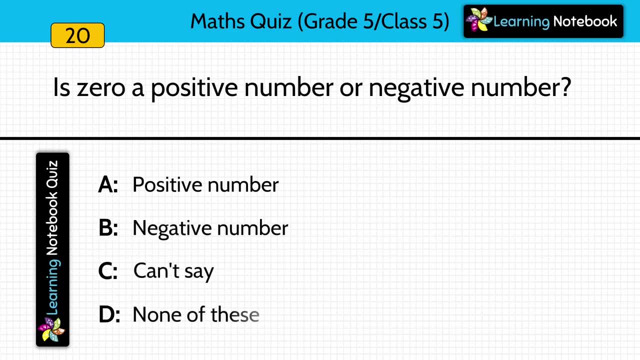 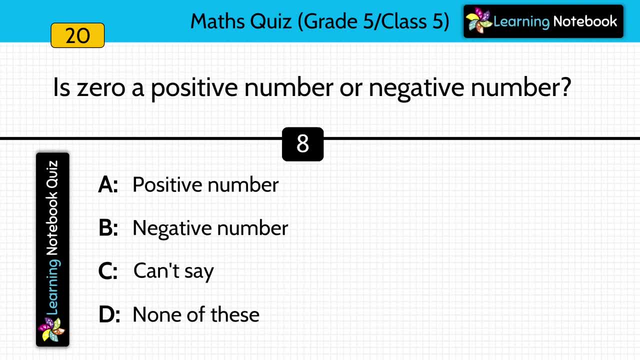 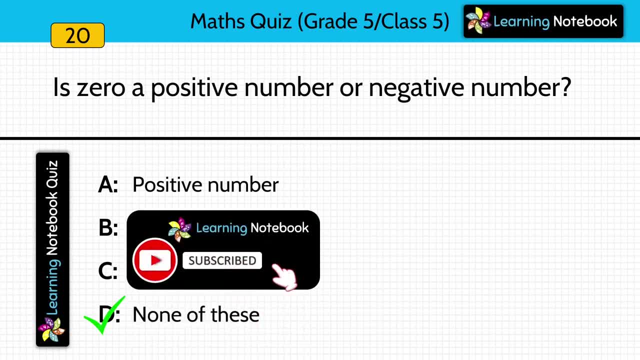 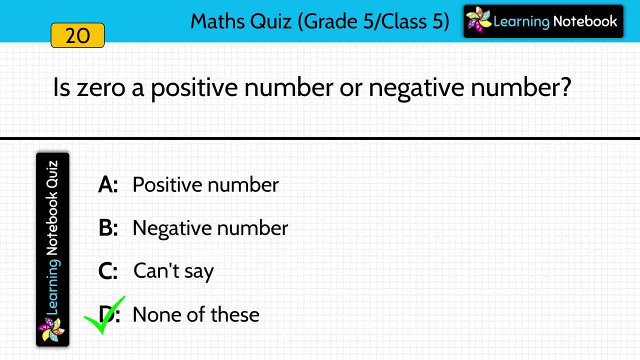 Is 0 a positive number or a negative number? Is 0 a positive number or a negative number? Answer is none of these. 0 is neither considered as a positive number nor a negative number. If you still not have subscribed to my channel: Learning Notebook. 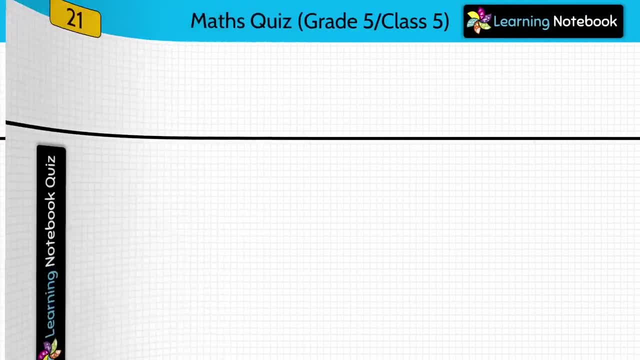 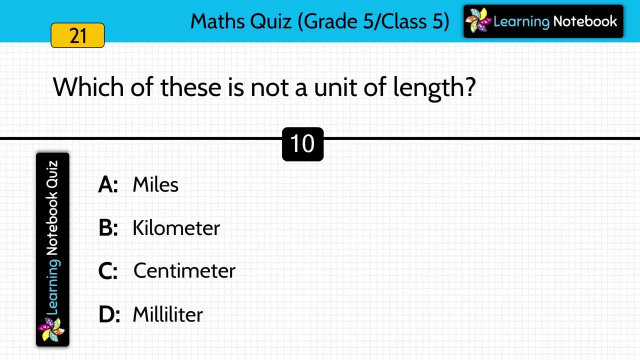 then do subscribe it right away. Which of these is not a unit of length? Unit of length Is it miles, kilometer, centimeter or milliliter? Answer is no. Answer is option D: milliliter. Milliliter is a unit of capacity. 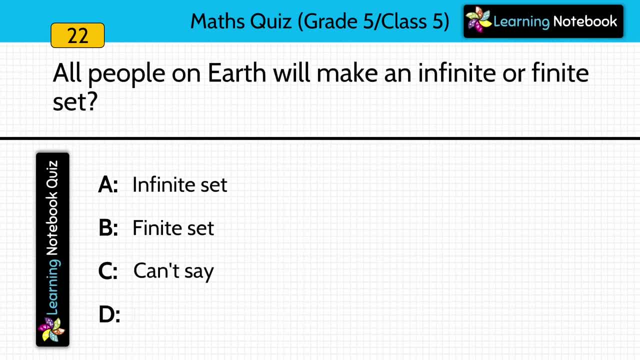 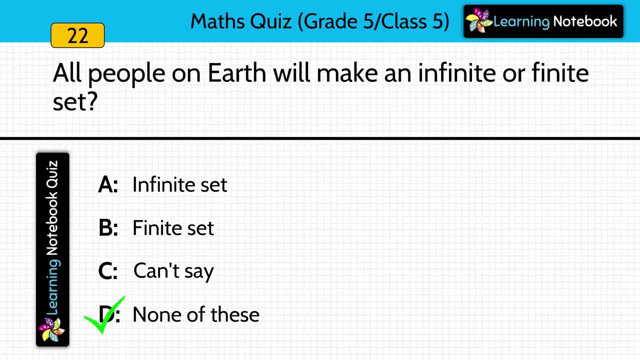 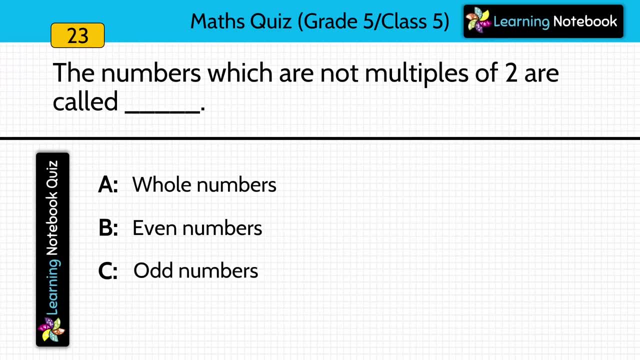 All people on earth will make an infinite or finite set. All people on earth will make an infinite or finite set. All people on earth will make an infinite or finite set. Answer is option D: none of these. The numbers which are not multiples of 2 are called dash. 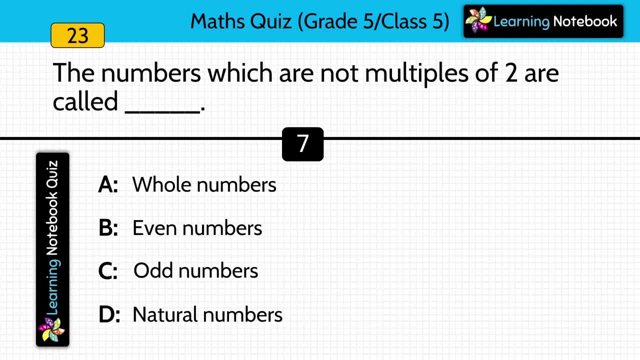 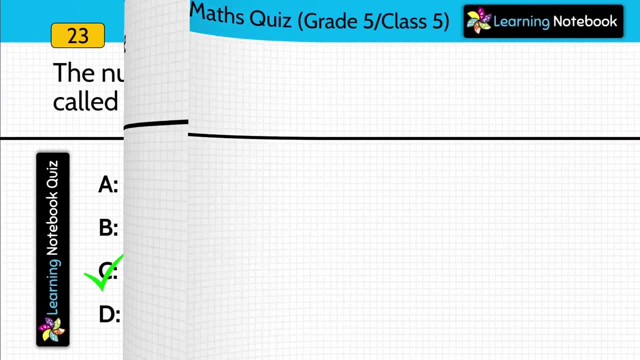 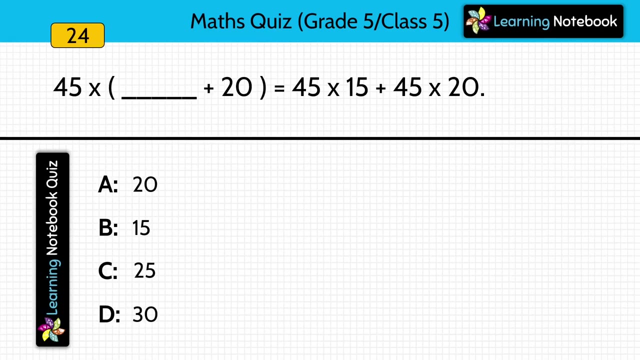 Numbers which are not multiples of 2, are they called as whole numbers, even numbers, odd numbers or natural numbers? Answer is option C, odd numbers. They are known as odd numbers. Solve this: 45 into brackets, dash plus 20 equals to 45 into 15 plus 45 into 20.. 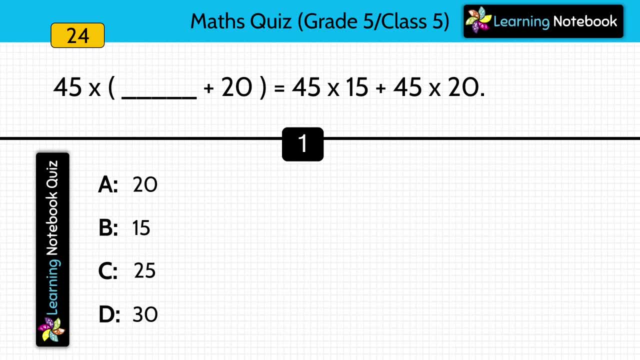 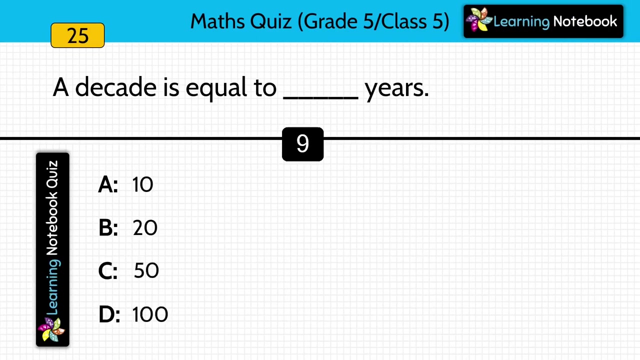 So what will come in this blank? Yes answer is 15.. 45 into 15 plus 20 equals to 45 into 15 plus 45 into 20.. A decade is equal to dash years. How many years are in a decade? 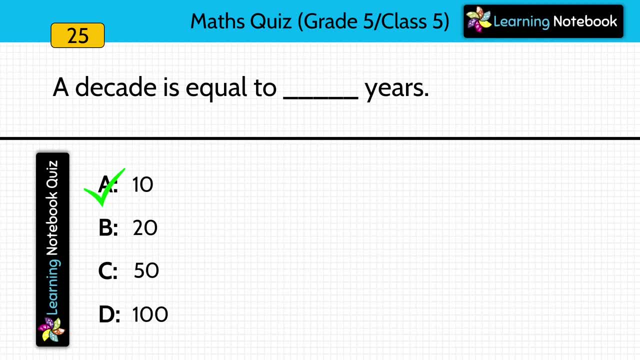 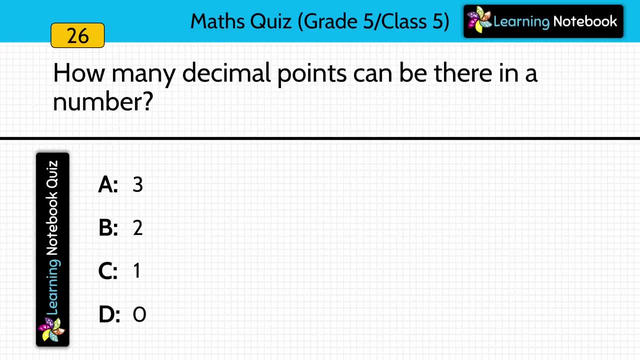 Answer is option A: 10 years. How many decimal points can be there in a number? How many decimal points Can be there in a decimal number- 3,, 2,, 1 or 0?? Yes, only one decimal point can be there in a number. 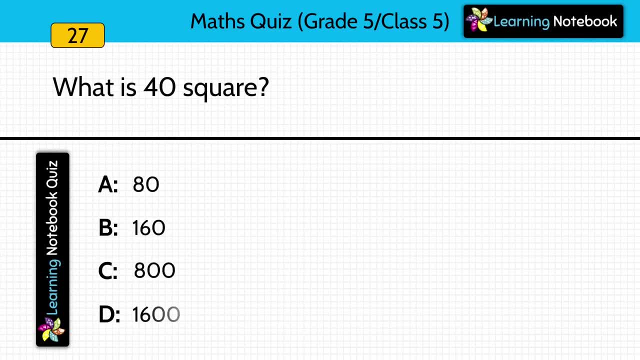 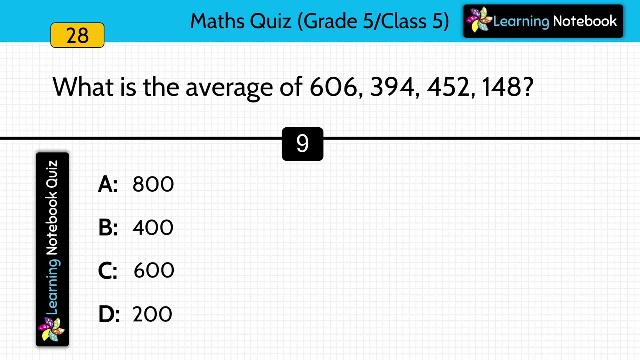 What is 40 square? Is it 80,, 160,, 800 or 1600?? Answer is option D, 1600.. Next question: What is the average of these four given numbers? You need to know how to find average of numbers. 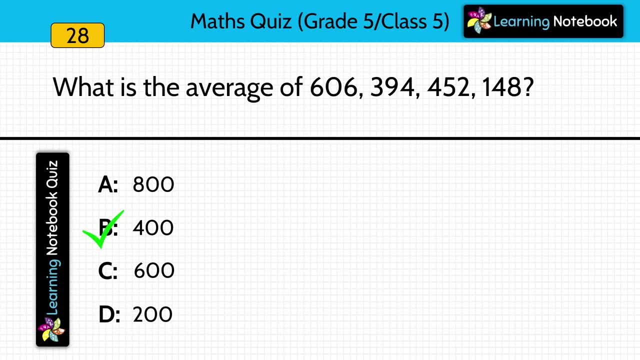 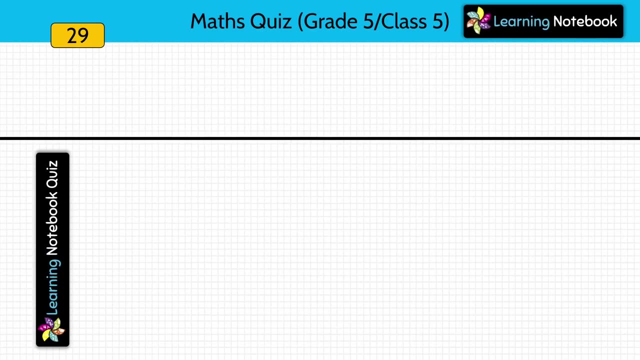 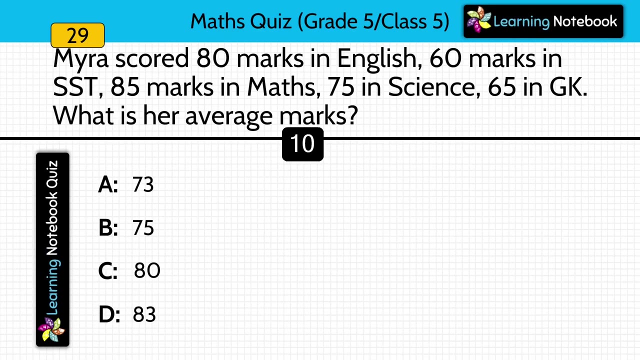 Answer is 400.. To find average of these numbers, first we will add all of them and then divide them by 4, because there are 4 numbers. So we get the answer as 400.. Next question: Myra scored 80 marks in English, 60 marks in SST, 85 marks in Maths, 75 in Science and. 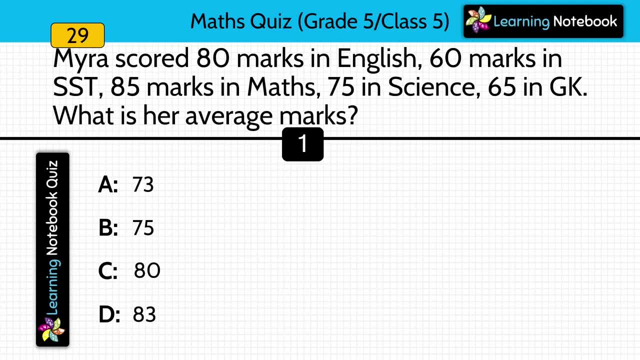 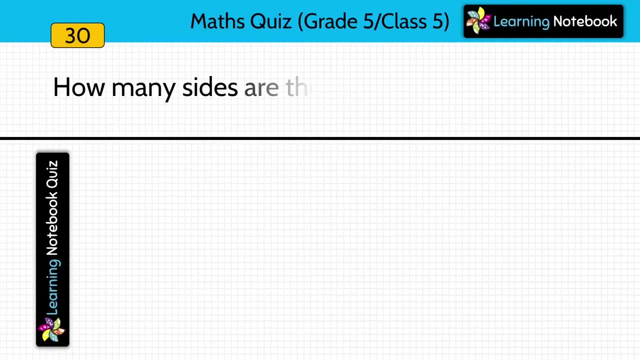 65 in GK. What is her average marks? Answer is 73.. We will find average marks by first adding all these numbers and then dividing them by 5, because there are 5 numbers. So we get the answer as 73.. How many sites are there in Pentadecagon? 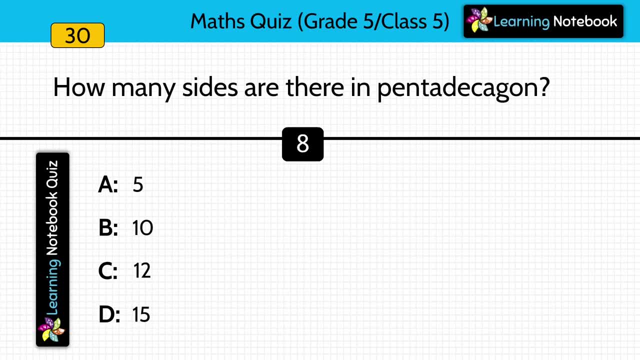 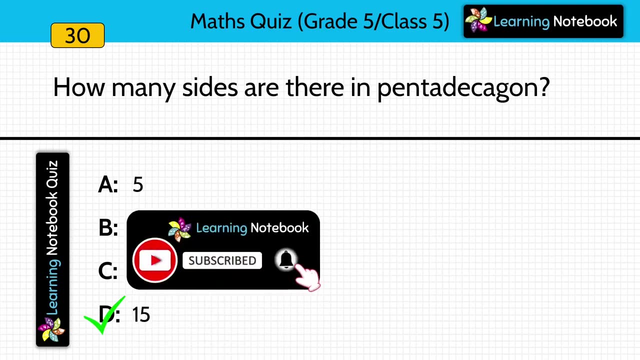 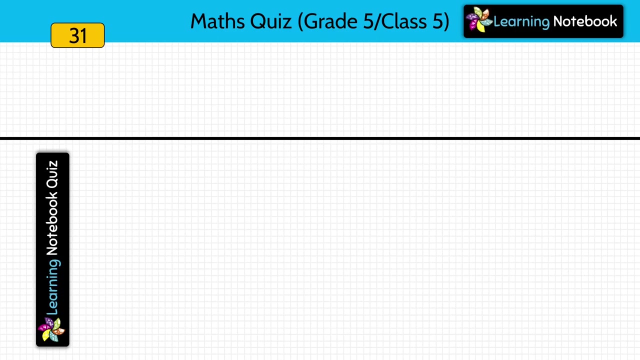 Do you know what is Pentadecagon? Yes, Do you know what is Pentadecagon? The answer is 15.. Pentadecagon has 15 sites. Let's see the next question: How many positive numbers are there between minus 7 and 7?? 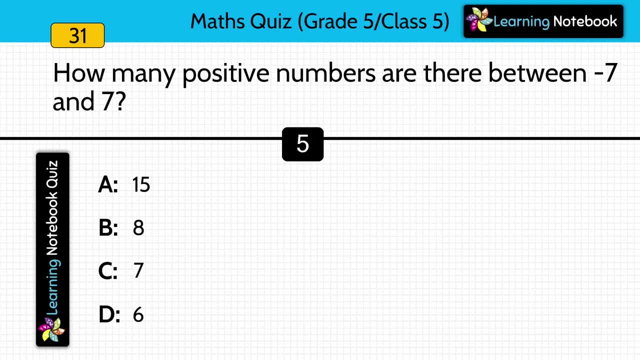 That is negative 7 and 7.. Positive numbers: Options: 15,, 8,, 7 or 6.. Answer is 7. There are only 7 positive numbers Because we know from negative 7 till negative 1, all are negative numbers. 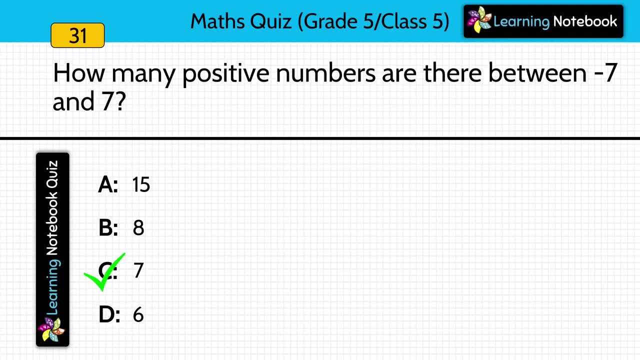 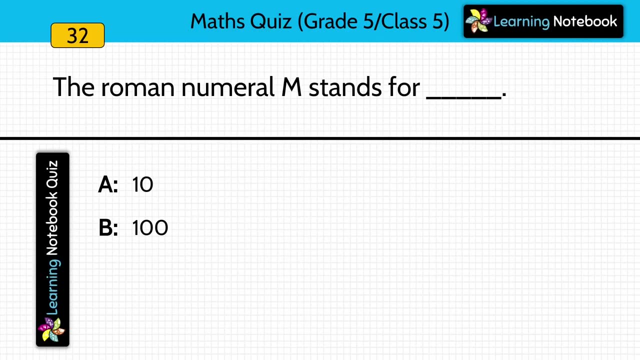 Then we have 0, which is considered neither as a positive number nor as a negative number, And then we have 1 to 7.. Only those numbers are positive numbers. The Roman numeral M stands for what? For which number Roman numeral M stands for? 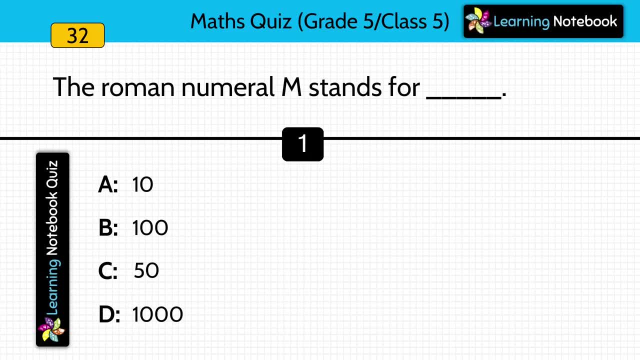 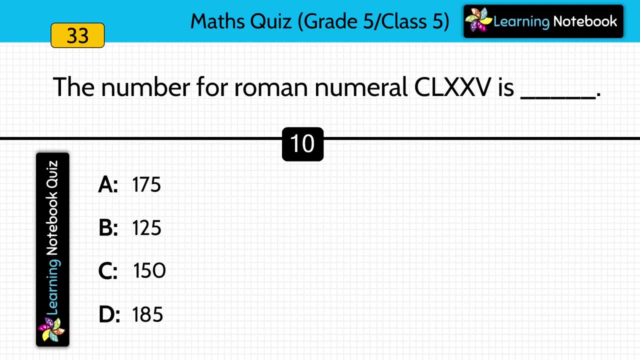 Is it 10, 150 or 1000?? Answer is 1000.. The number for Roman numeral CLXXV is dash. For this. you should know which symbol stands for what number. Answer is 175.. How did we find this? 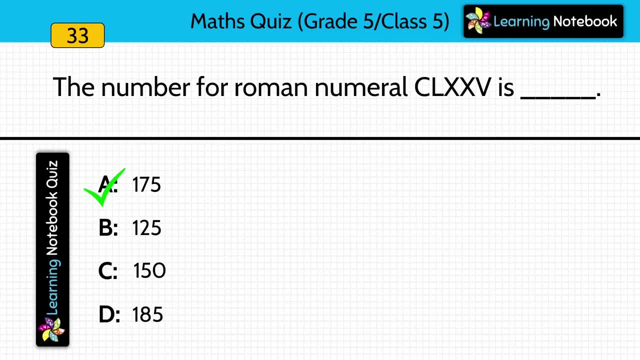 Because we know Roman symbol C stands for 100.. L equals to 50. X means 10 and V stands for 5.. So we have added these numbers and we have got the answer as 175.. Next question: This is the given statement. 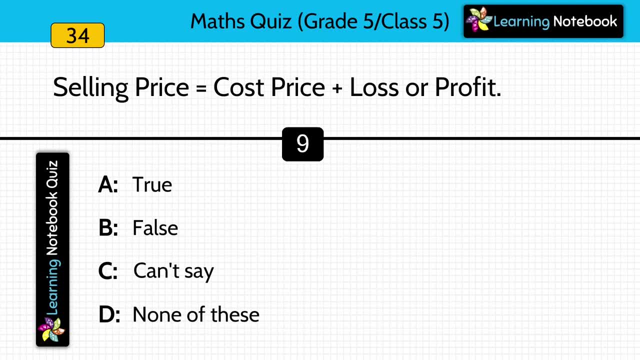 Selling price equals to cost price plus loss or profit. Is it true, false, can't say, or none of these. The answer is false because selling price equals to cost price plus profit. It is not equal to cost price plus loss, So this is false. 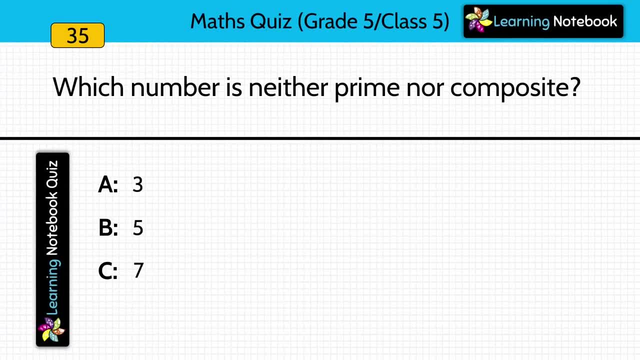 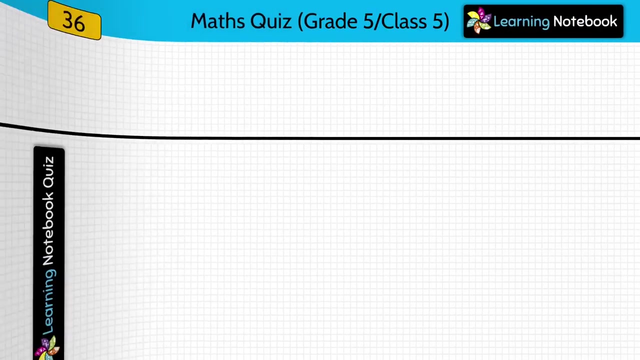 Which number is neither a prime number nor a composite number? Look at the options 3,, 5,, 7 or 1.. Answer is option D 1.. It is considered neither as a prime number nor as a composite number. Next question: 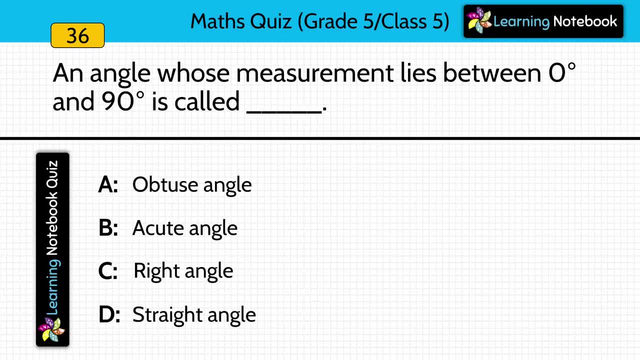 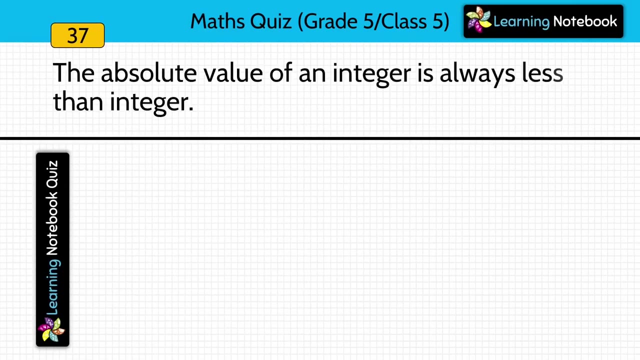 An angle whose measurement lies between 0 degree and 90 degrees is called dash Options. Is it obtuse angle, acute angle, right angle Or straight angle? Answer is acute angle. Such angle is known as acute angle. The absolute value of an integer is always less than integer. 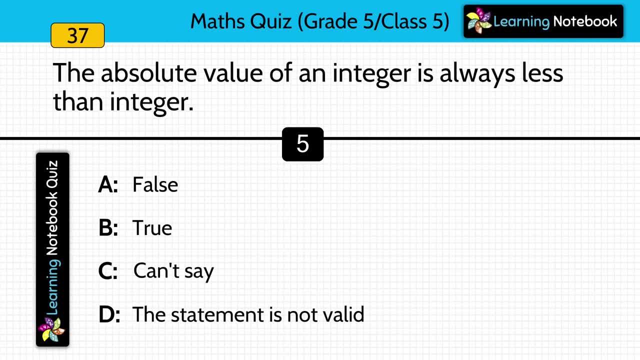 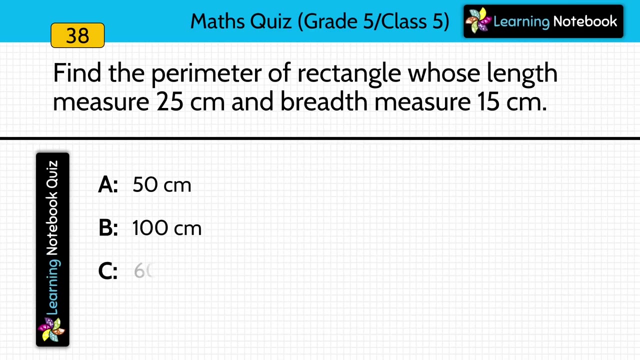 Is this statement false? true, can't say. or this statement is not valid. Answer is false, Because the absolute value of an integer is always greater than that integer. Find the perimeter of rectangle whose length measures 25 cm and breadth measures 15 cm. 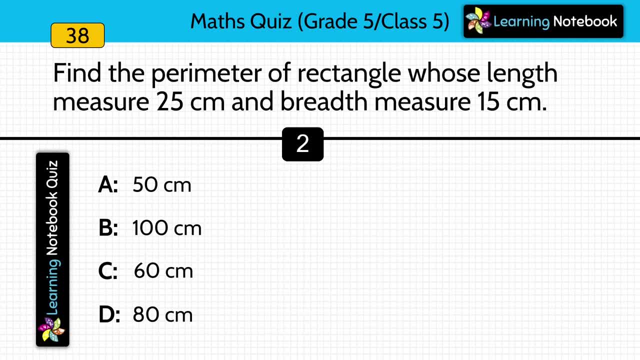 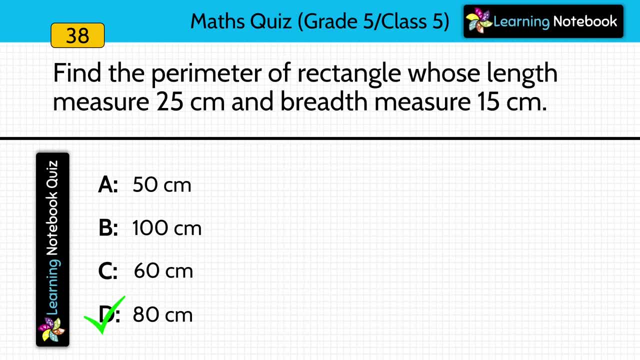 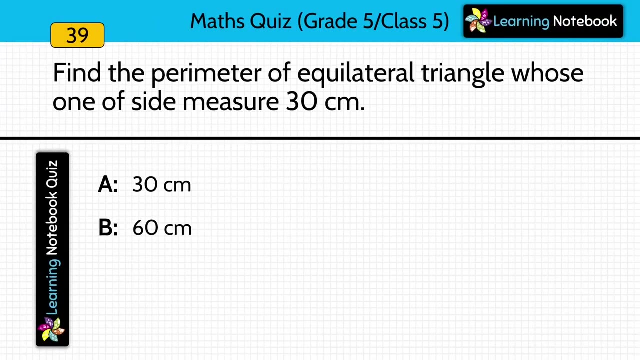 How did we solve this? We know perimeter of rectangle equals to twice into length plus breadth. So length is 25 plus 15 equals to 40. So 2 into 40 equals to 80.. Next find the perimeter of equilateral triangle. 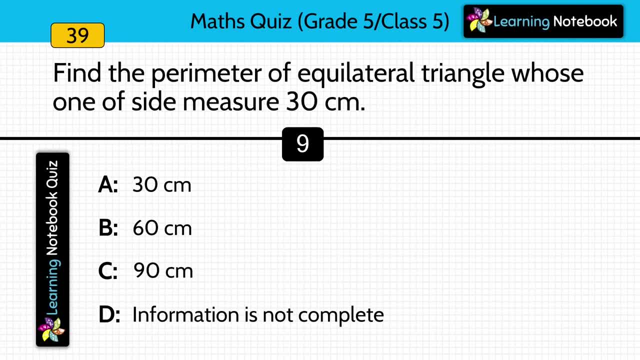 whose one of the side measures, whose one of the side measures 30 cm. Do you know what is equilateral triangle? It is a triangle which has all the sides equal. So if we are given with one side which measures 30 cm, 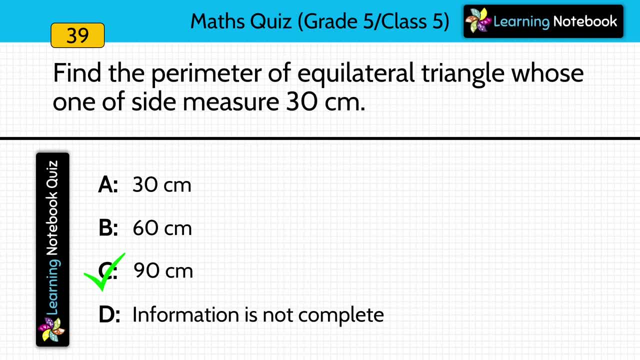 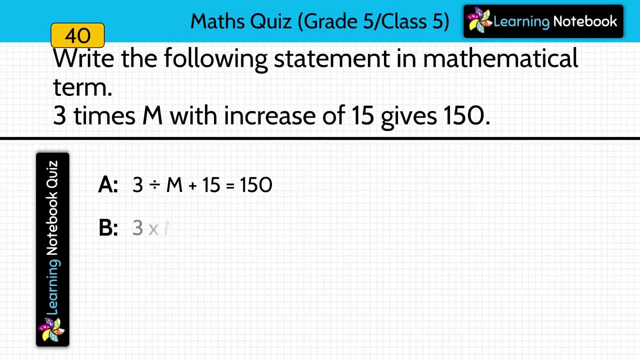 it means rest of the two sides also measures 30 cm, So perimeter of equilateral triangle will be 30 plus 30 plus 30, which is equals to 90 cm, So it will be 50.. Write the following statement in mathematical terms: 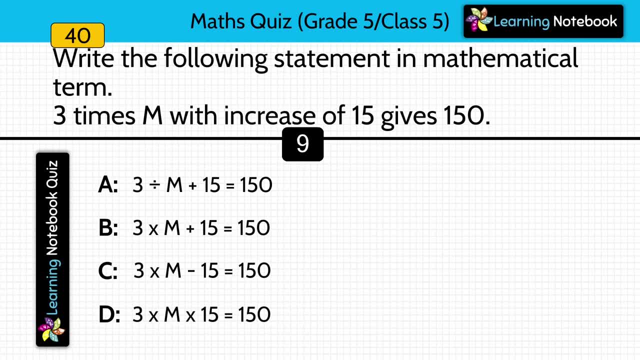 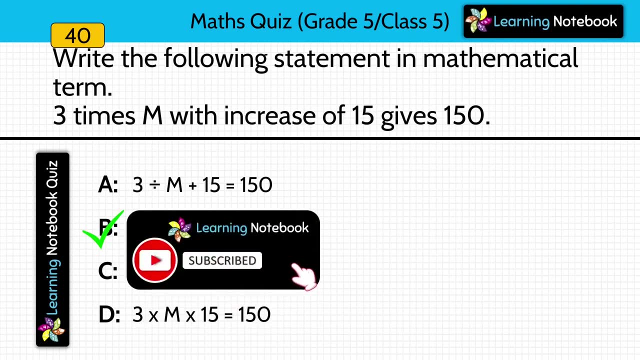 Write the following statement in mathematical terms: 3 times m with increase of 15 gives 150.. 3 times m with increase of 15 gives 150.. Answer is option B, 3 into m, because 3 times m means 3 multiplied by m. 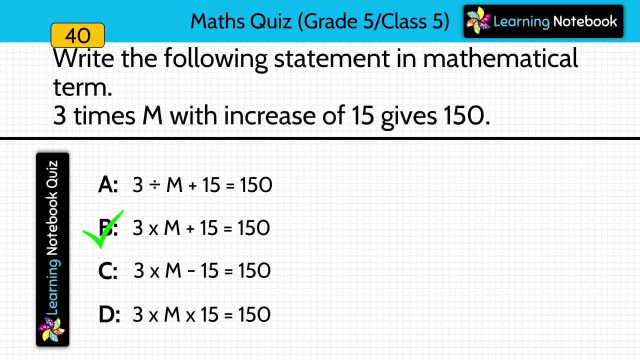 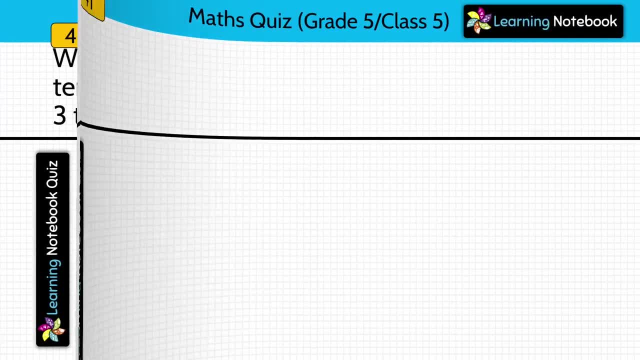 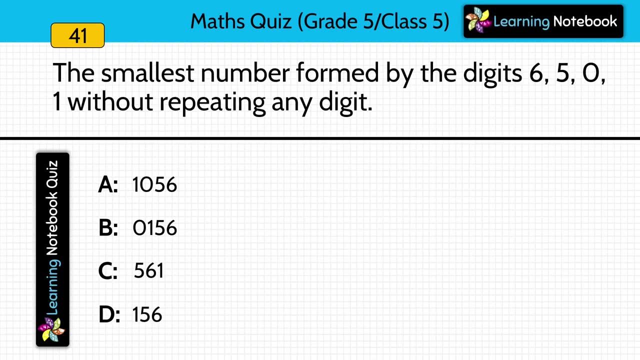 With increase of 15 means 3 multiplied by m plus 15 and gives 150 equals to 150.. So this is our answer. Next question: the smallest number formed by the digits 6,, 5,, 0 and 1, without repeating. 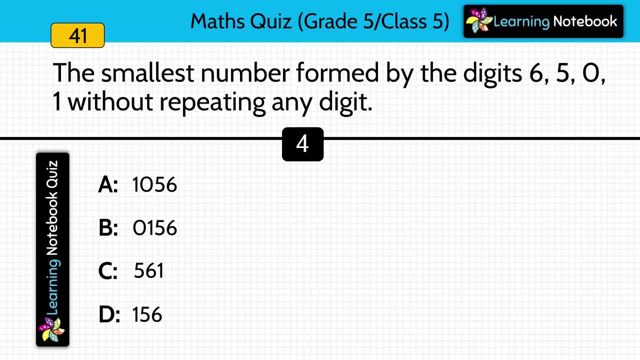 any of these digits. You need to form the smallest number using these four digits. Answer is 1056.. Now you must be thinking: why can't we write 0156? because we know that 0 is the smallest number, So why can't we start with this digit, 0?? Students, when we 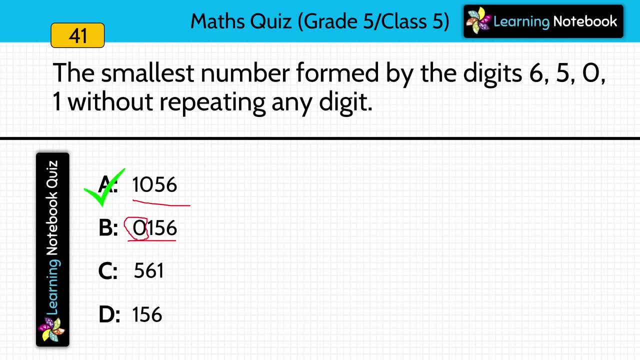 start any number with 0, then this 0 doesn't hold any value. 0156 is nothing but 1556.. Okay, So here in this number, in 156, we haven't used 0 and we have to use all these. 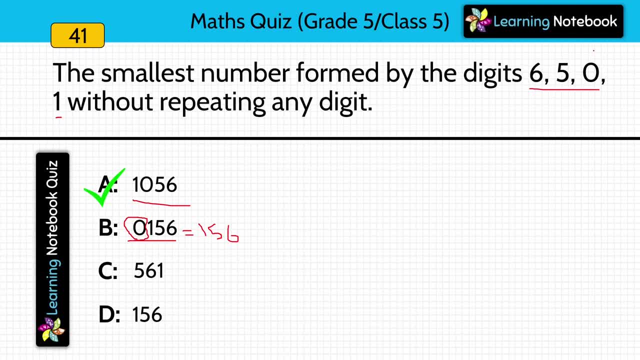 digits. So whenever you are given with digit 0 and you have to form the number, so that you have to form the smallest number, then that 0 should be at second place here. So we will start with the next smallest digit, which is 1,, then we will write 0,, then 5,. 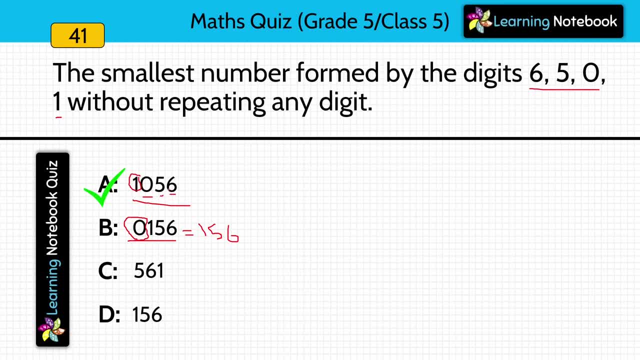 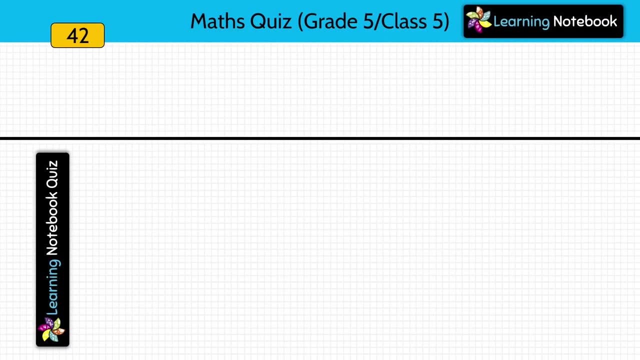 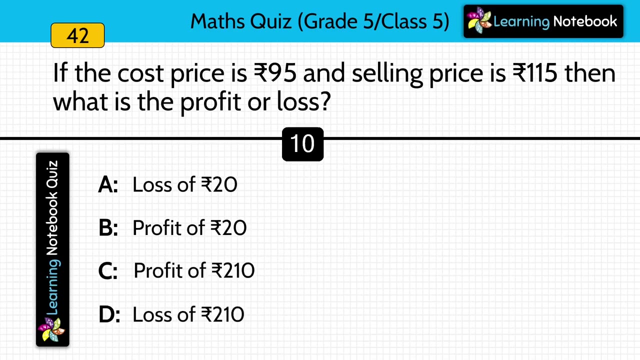 and then 6 in ascending order we have written. So in this way, we have formed the smallest number using all these four digits, and we haven't repeated any digit as well. Okay, Next question: if the cost price is Rs 95 and selling price is 115, then what is the? 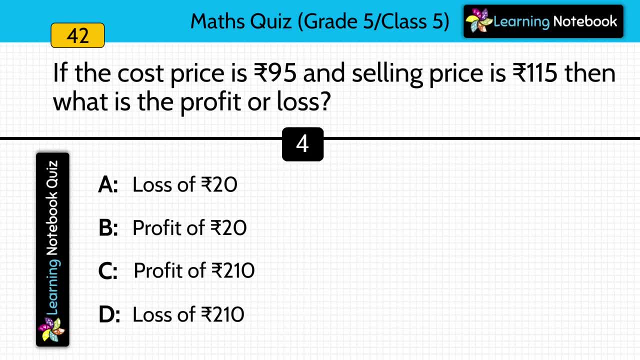 profit or loss? Yes answer is profit of Rs 20 because selling price is greater than cost price. So we will do 115 minus 95, which is equals to 20, and that is profit of Rs 20.. Brick is an example. 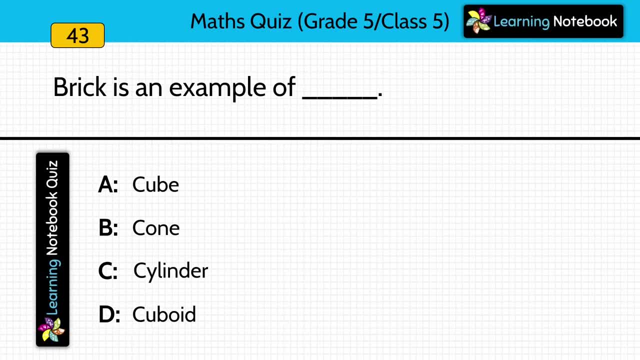 of dash. Is it an example of cube, cone, cylinder or bar? Yes, answer is profit of Rs 20.. So it is an example of cuboid? Yes, it is an example of cuboid. Average of first four odd. 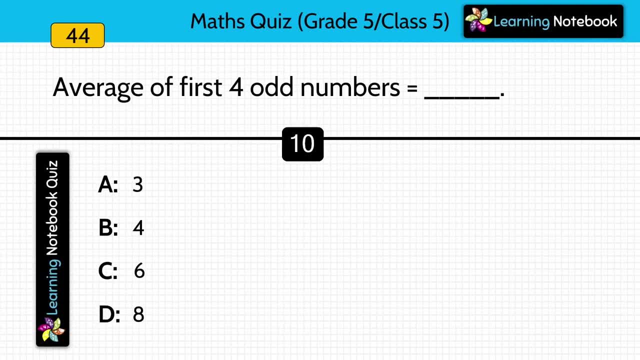 numbers. So here you have to tell the average of first four odd numbers. So quickly think about the first four odd numbers. Answer is 4.. How did we find this? First of all, think of first four odd numbers. These: 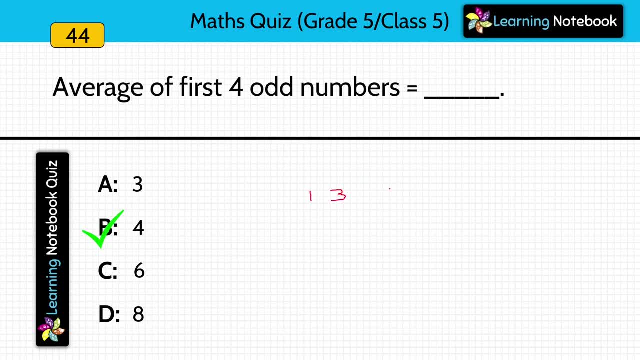 are 1,, 3,, 5,, 7.. Now add all of them. 1 plus 3 is 4,. 4 plus 5 is 9, 9 plus 7 equals to 16.. Now divide this 16 by these count of numbers. These are 4.. So 16 divided by 4 equals to: 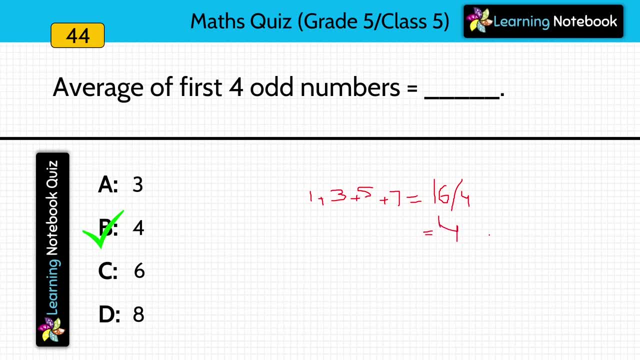 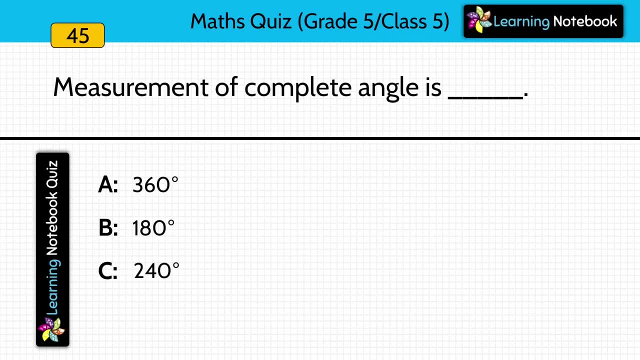 4.. So this is our answer, 4.. Let's see the next one: Measurement of complete angle. is dash, You have to tell the measurement of complete angle. Yes, Yes, Yes, Yes, Yes, Yes. Answer is option A: 360 degrees is the measurement of complete angle. 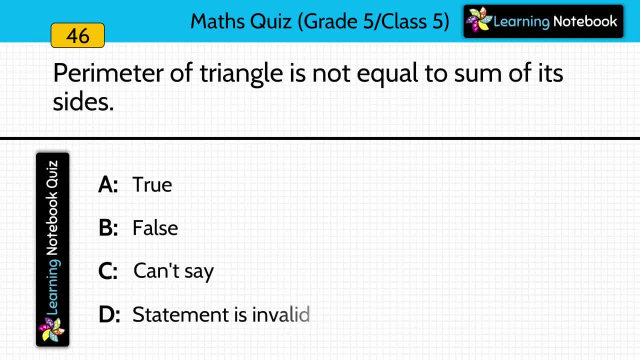 Perimeter of triangle is not equal to sum of its sides. Is this statement true or false? Or can't say, or the statement is invalid. Answer is false. This statement is false because perimeter of a triangle is equal to sum of its 3 sides. 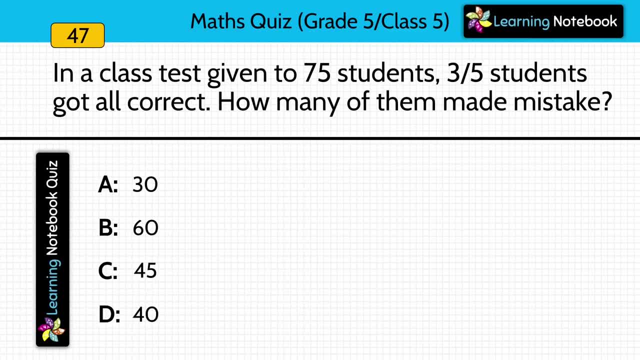 In the class test given to 75 students, 3 by 5 students got all correct. So how many of them made mistake? The answer is option A: 30.. So how did we find this Here? it is given that 75 students are there and 3 by 5 students got all correct. 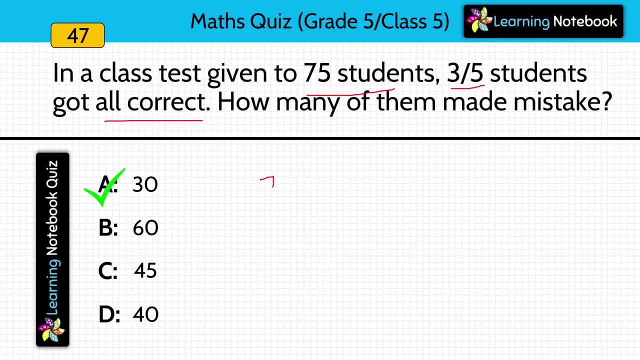 So first of all, let's find how many students- number of students- got all the- you know the entire test correct. So we are going to find out the number of students got all correct. So we are going to find out the number of students got all correct. 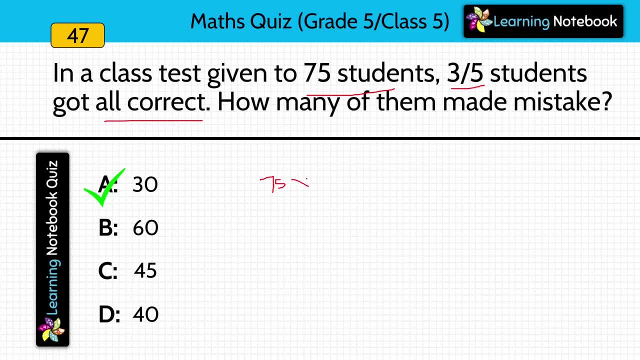 So we will do 75 into 3 by 5, let's simplify this: 5, 15 is 75. So now we have got 15 into 3, which is equals to 45. So 45 students got all correct. 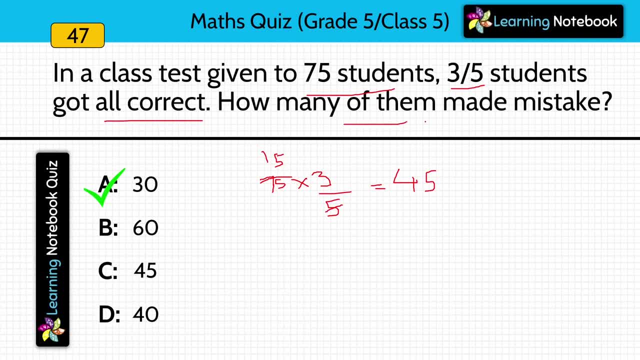 They have got the entire test correct And we have to find how many of them made mistake Now. we can easily find this by subtracting 45 from 75.. 75 is total number of students and 45 is the number of students which got all correct. 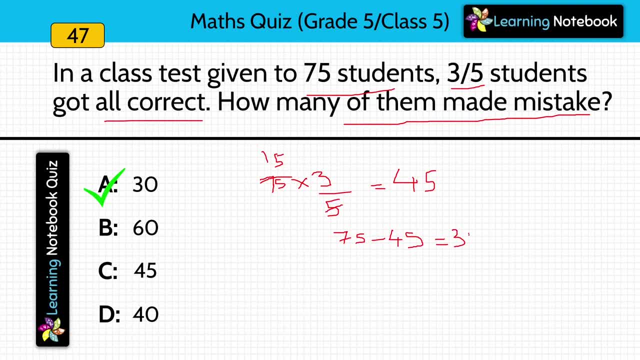 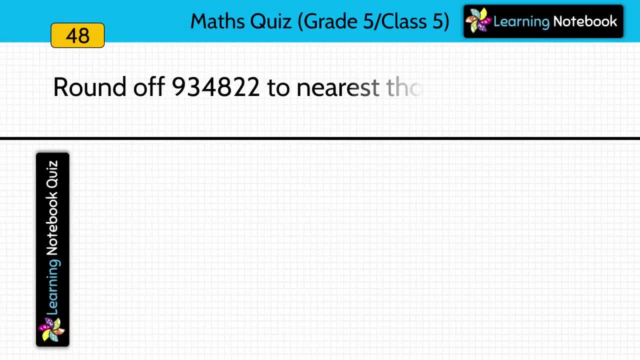 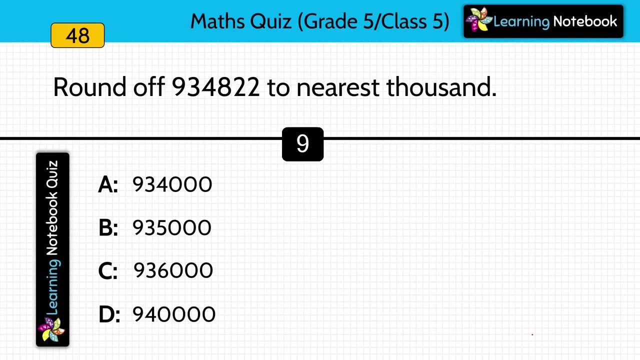 So 75 minus 45 is 30.. So this is how we will calculate this question. Next question: round off this number to nearest 1000.. You are given with this number And you have to round it off to nearest 1000. 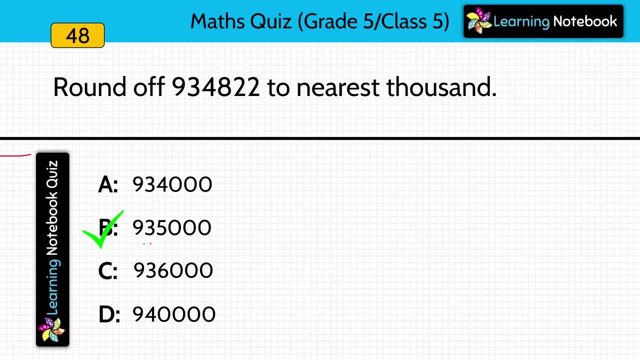 Answer is: what is the answer? 9,, 3,, 5,, triple 0.. Students remember to round off a number to nearest 1000, we look at its 100 digits. So here 100 digits is 8.. 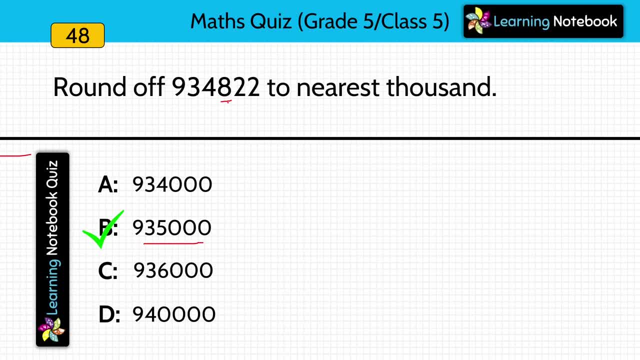 And since 8 is more than 5, we will round off this number. So we will round off this number to you know, to upwards 1000.. So, upwards 1000 or 4822 will be 5000. 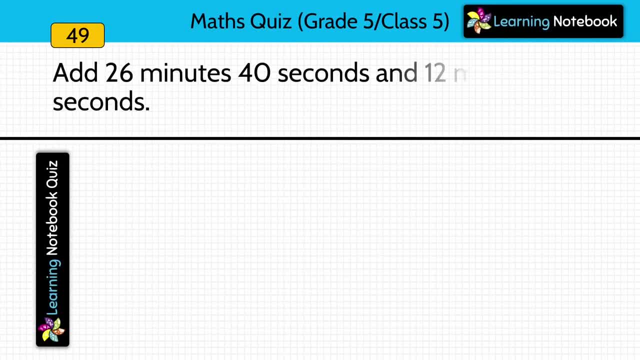 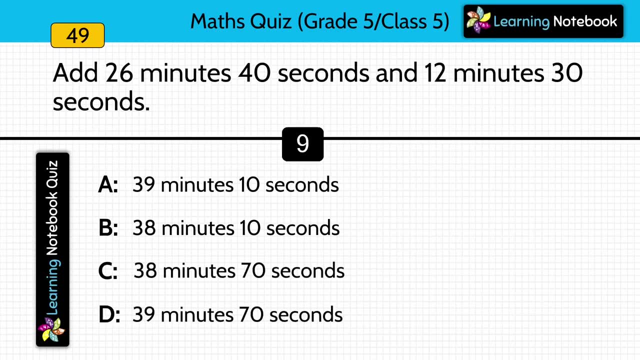 Okay, Next one: add 26 minutes 40 seconds and 12 minutes 30 seconds. Answer is option A. Answer is option A. Answer is option A: 39 minutes 10 seconds. So, students, how did we solve this? 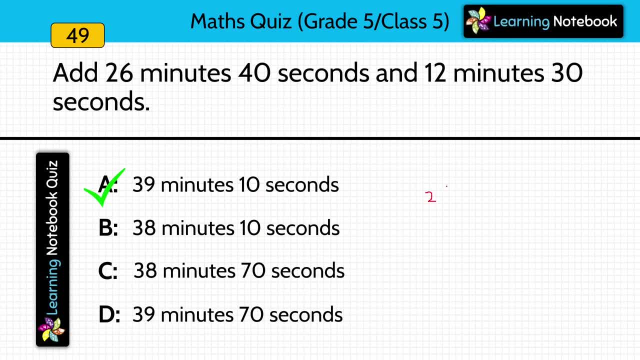 To solve this. first we will write the given numbers: 26 minutes, So we will write it under minutes column. And here we have seconds. I will write 40 here Now to write this: 12 minutes, 30 seconds. again we will write minutes under minute column. 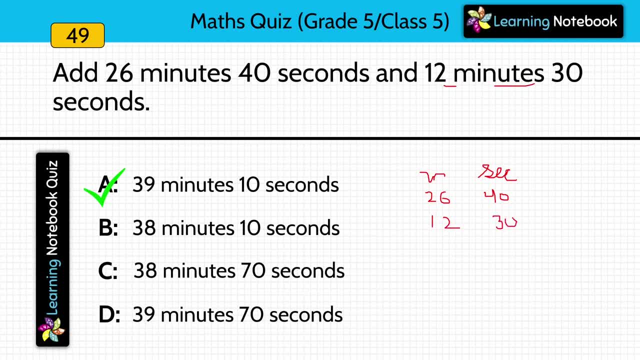 and seconds under seconds. Now let's add: 0 plus 0 is 0,, 4 plus 3 is 7.. Now, students, look here: 4 plus 3 is 7.. So we will get 70 here, 70 seconds. 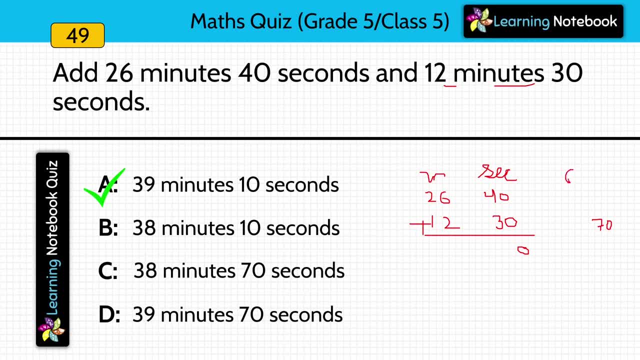 Now we know that 60 seconds- this 60 seconds- equals to 1 minute, right? So instead of writing 70 here, we will do 70 minus 60, this 60, which is equals to 1 minute, will be carried over here. 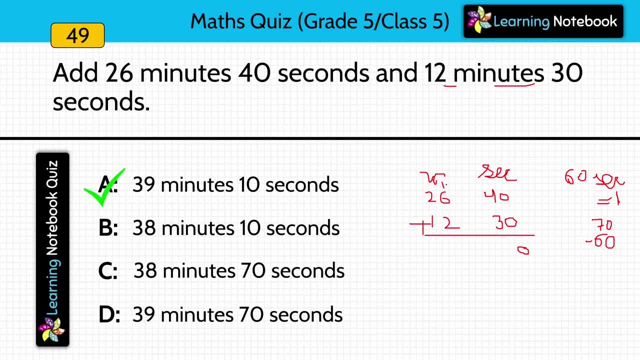 I have carried over 1 minute here in this minute column, Okay, And I will subtract 60 from here because I have taken out 1 minute. So 70 minus 60 is 10.. So this is what I am going to write here: 10 instead of 70, because we know that in 70. 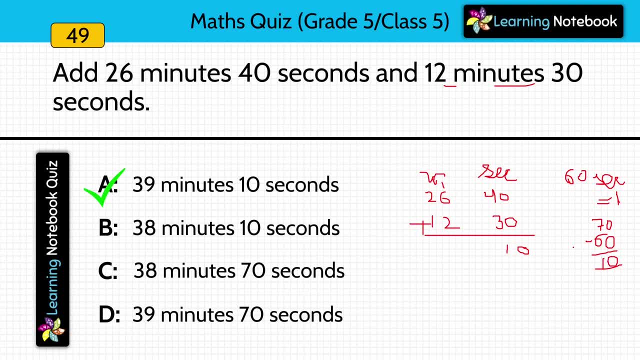 seconds. there are 60 seconds involved, So we will take out 60 seconds, which is equals to 1 minute, and we will carry it here 1.. Okay, Now let's add minutes. 1 plus 6 is 7, 7 plus 2 is 9 and 2 plus 1 is 3..